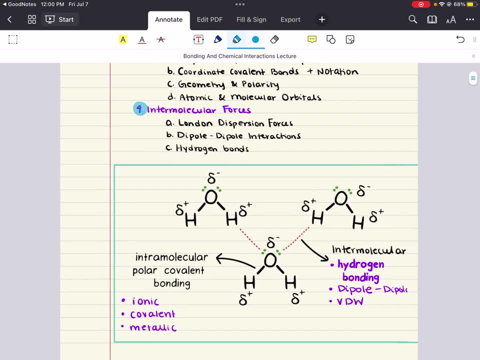 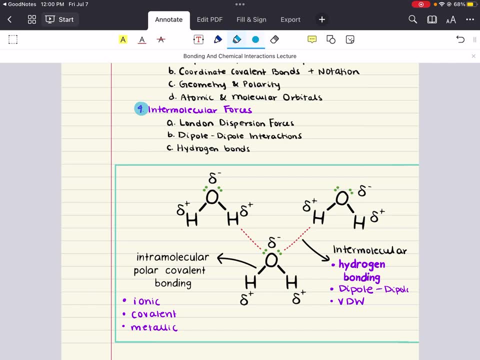 intermolecular forces. The hopes is to be able to understand behavior of covalent and ionic bondings, as well as reviewing a system by which the bonding of electrons are accounted for through Lewis structures, as well as identifying and addressing the main principles of things like VSEPR theory, atomic versus molecular orbitals and also the 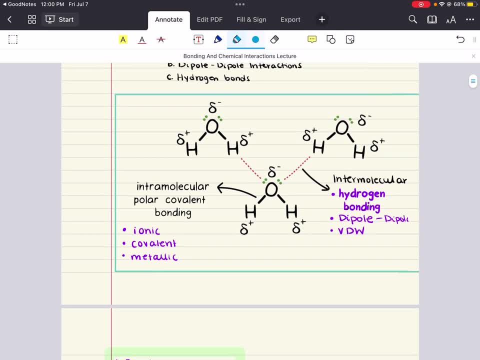 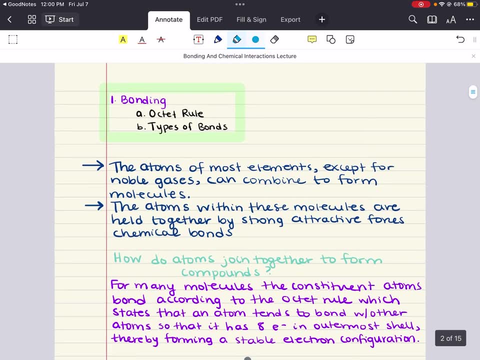 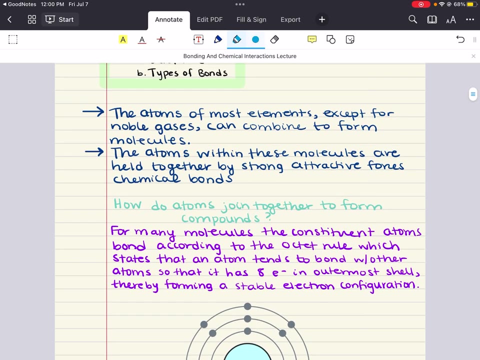 various modes of interactions between molecules, aka intermolecular forces. By the way, we're going to go ahead and start with our first objective. We're going to discuss bonding Now. when atoms of most elements come together, they can form molecules. These: 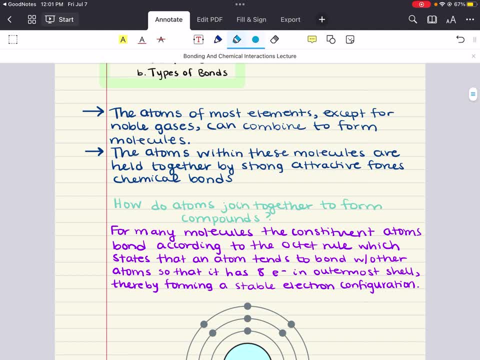 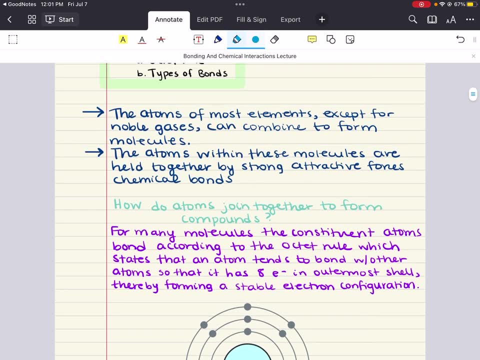 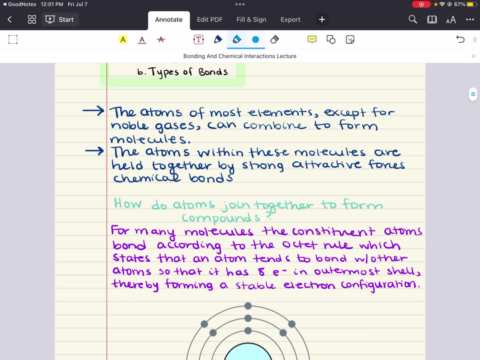 molecules are held together by something called chemical bonds, which are formed when the valence electrons of the atoms interact with each other, And so this allows us to make our first very important point here. It is those outermost electrons of atoms that are going to be participating in chemical bonding, Those 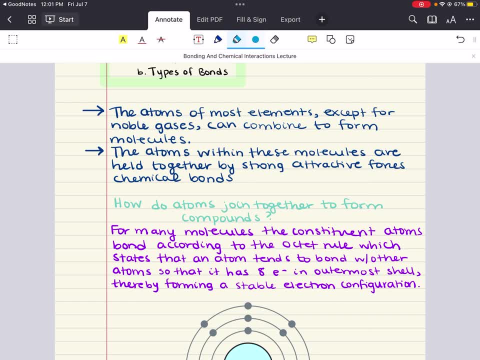 innermost electrons, the ones that are closest to the nucleus, are not going to be participating in bonding, And so when we talk about chemical bonding, we're talking about valence electrons, the interactions of valence electrons, of the elements that are coming together to form. 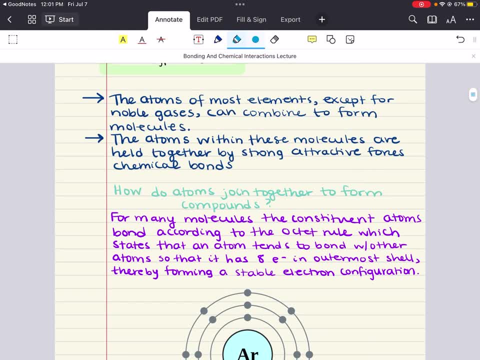 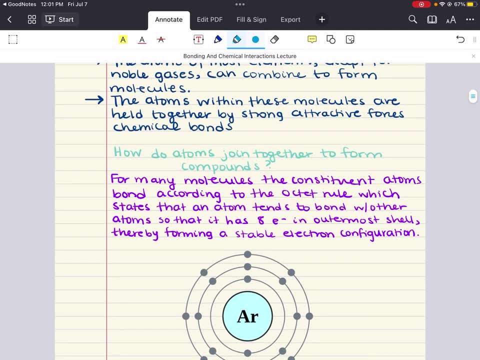 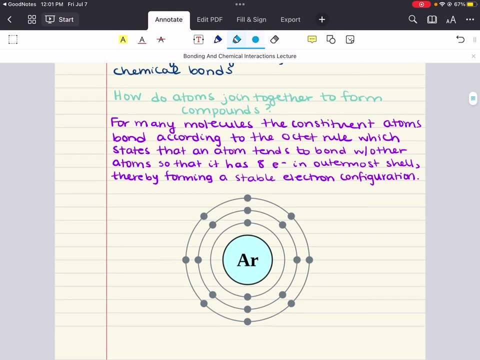 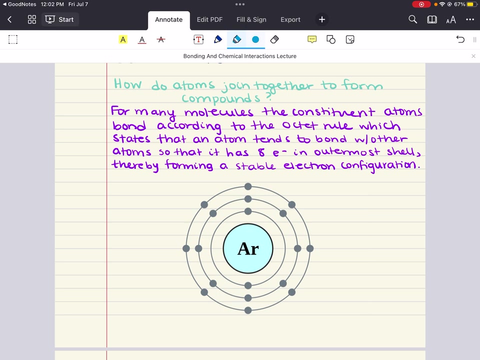 chemical bonds. The interesting thing is that the properties of these new compounds are usually very different from the properties of individual atoms, And so that allows us to probe further. How do atoms join together to form compounds? For many molecules, the constituent atoms bond according to the octet rule. All right, 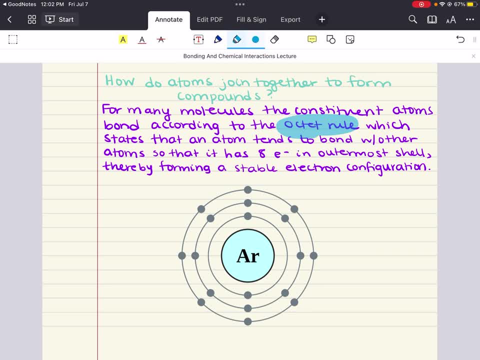 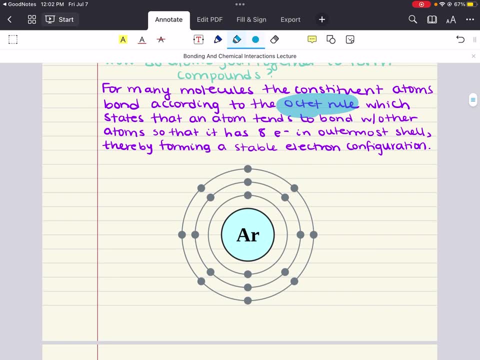 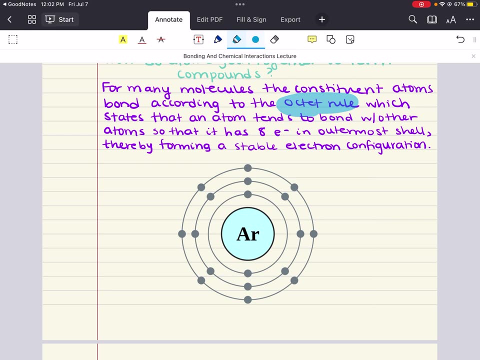 bond according to this octet rule. What is the octet rule? Well, the octet rule states that an atom tends to bond with other atoms so that it has eight electrons in its outermost shell, thereby forming a stable electron configuration that's very similar to that of noble gases. all right, 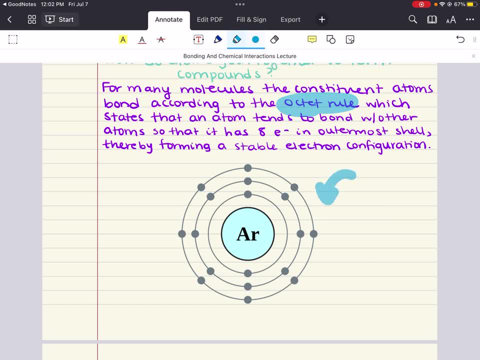 One example of a noble gas is argon. all right, We see the Lewis dot structure of argon and we're going to learn how to draw Lewis dot structures for atoms here really soon. but let's just look at this, all right. 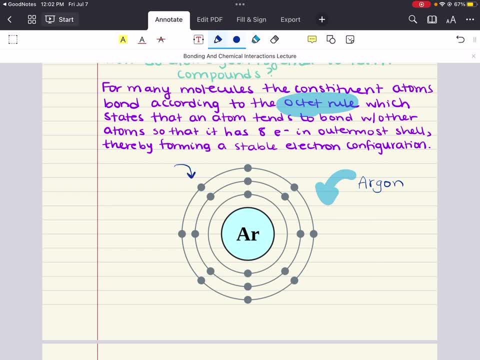 Here's argon, and let's look at its outermost valence electrons. all right, We have one, two, three, four, five, six, seven, eight electrons. There are eight electrons in the outermost shell of argon. 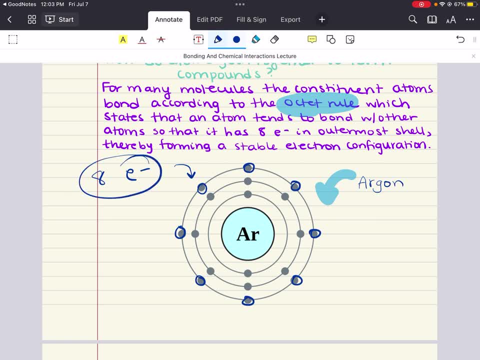 Argon is a noble gas. It has these eight electrons. This is considered a stable electron configuration. The noble gases: if you look at row eight on the periodic table, those noble gases, they all have eight valence electrons in their outermost shell. 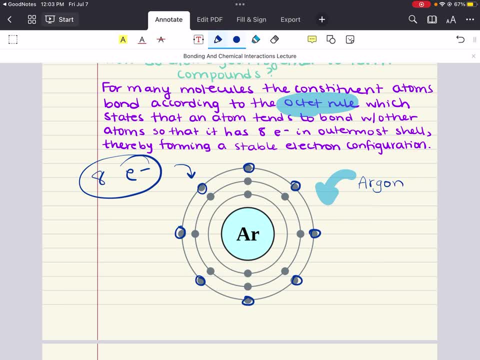 and this is referred to as a stable electron configuration and we talk about the octet rule. in relation to noble gases, We state that an atom tends to, It tends to bond with other atoms so that it can have, so that it can reach this eight-electron configuration in its outermost shell. 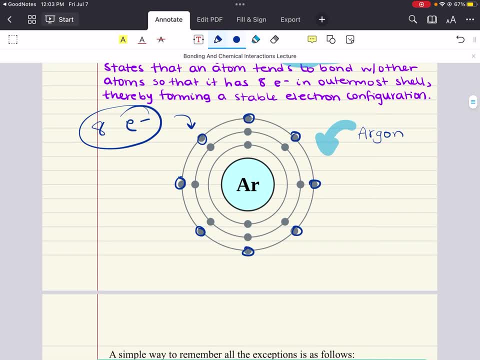 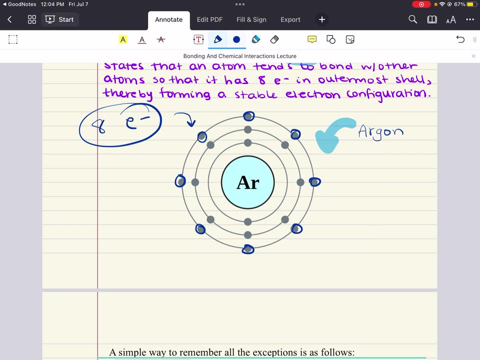 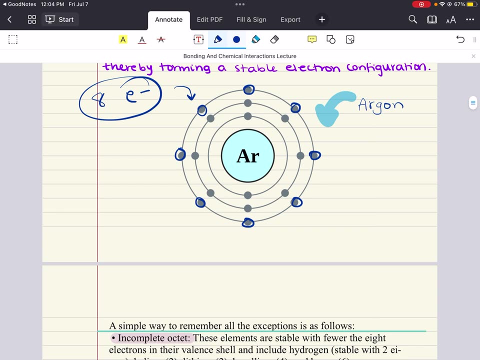 and so then it becomes stable. Therefore, this is kind of a rule of thumb that we talk about. all right, But that's what it is. all right. It is just more of a rule of thumb because there are more elements that can be exceptions to this rule. 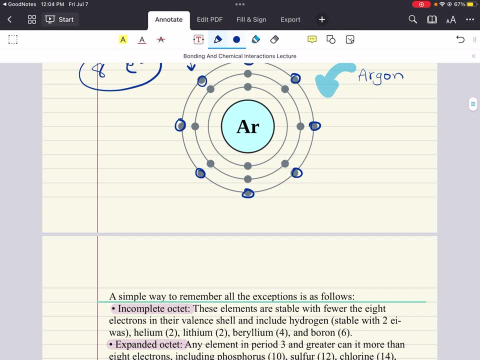 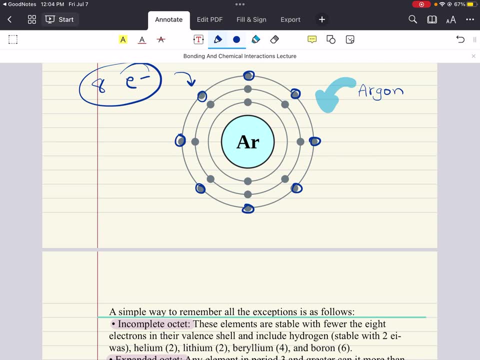 than there are elements that can be exceptions to this rule. So let's look at this. Let's look at this. These exceptional elements include things like hydrogen, which can only have two valence electrons, and that is its stable electron configuration. 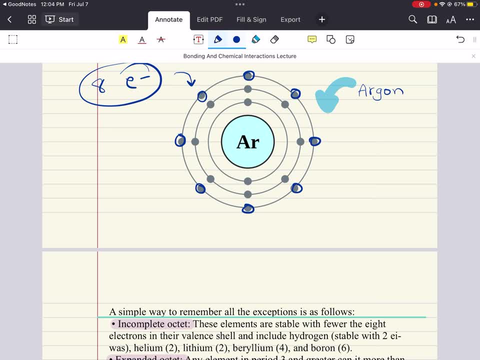 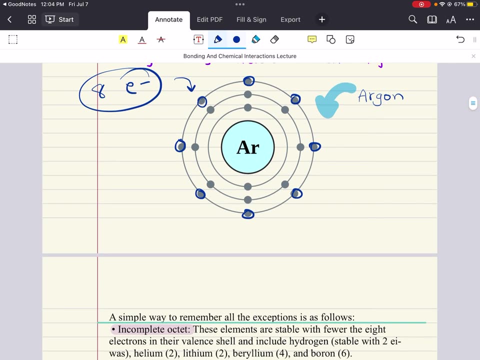 It achieves that configuration of helium when it has those two electrons in its outermost shell. Lithium and beryllium are also exceptions to the rule. They bond to attain two and four valence electrons respectively. Boron is another good example of an exception. 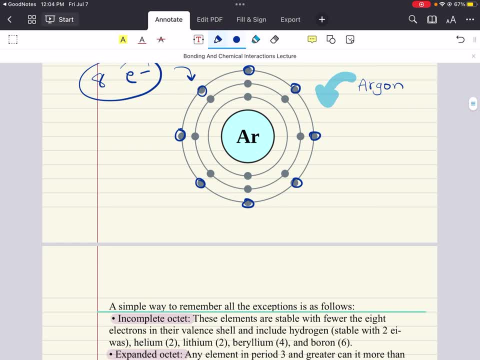 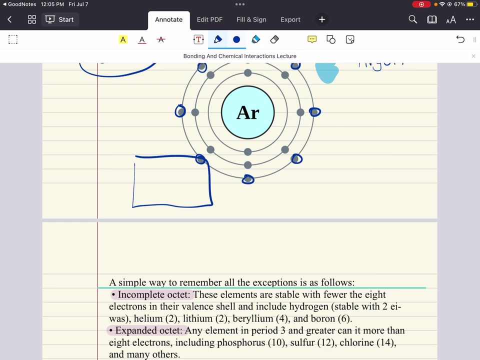 It bonds to attain six valence electrons And also all elements in period three and greater, those transition elements, transition metal elements. they can be exceptions to this rule and they can expand the valence shell to include more than eight electrons by incorporating those d orbitals. 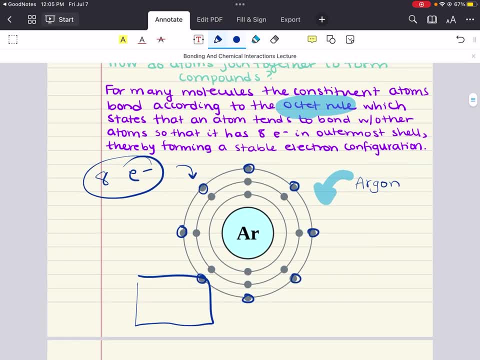 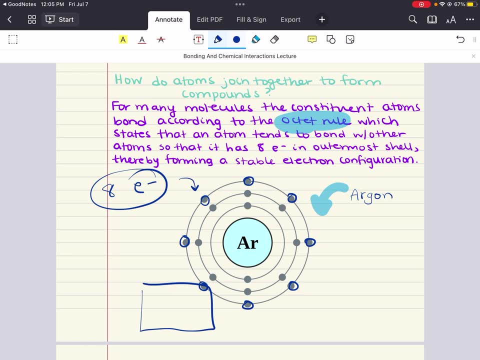 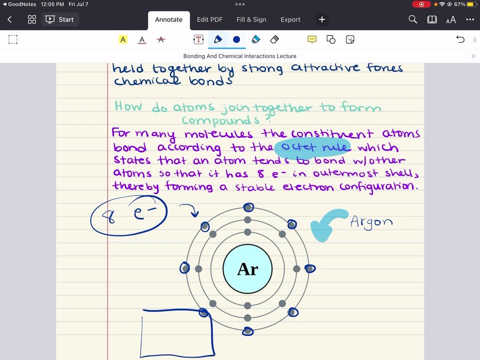 All right, So we've kind of said two things here that can be contradicting to a student who's learning this for the first time. right, We said that for many molecules, the constituent atoms, they bond according to the octet rule. They bond in a way to help meet this so-called octet rule. 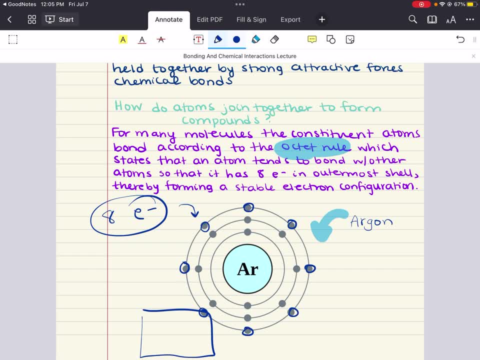 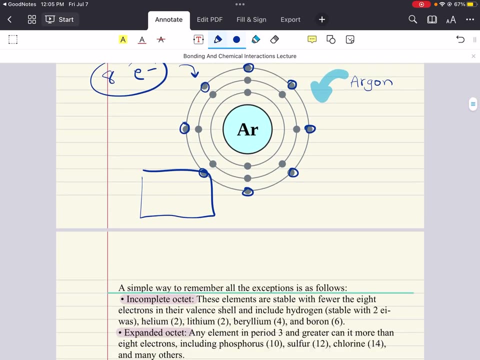 to help reach this eight electron valence, these eight electrons in their outermost shell, All right. And then they're comparable to noble gases, And this is referred to as a stable electron configuration. But to this we also have to add that there are exceptions to this rule. 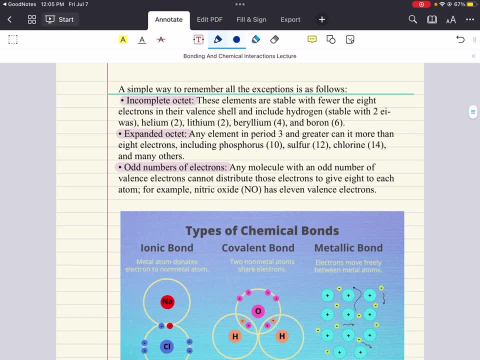 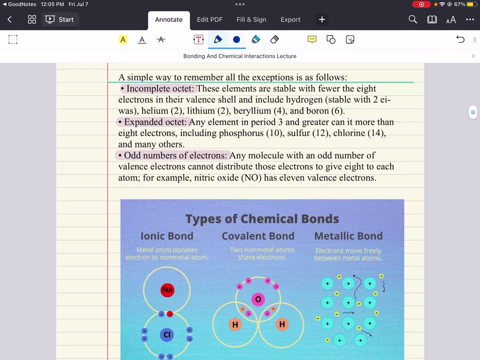 And we need to be able to navigate the realm of exceptions to this octet rule. And so how do we keep track of these exceptions? Well, three rules to keep in mind that will help us with this. All right, We have our first rule. 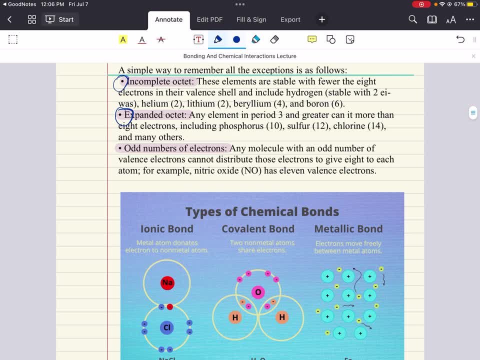 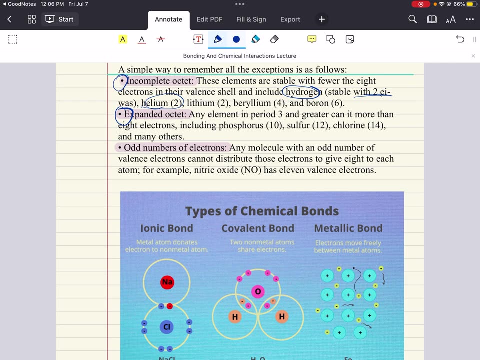 This incomplete octet. These elements are stable with fewer than eight electrons in their valence shell And they're going to include hydrogen, which is stable with two electrons. It includes helium, which is stable with only two valence electrons. It includes lithium. 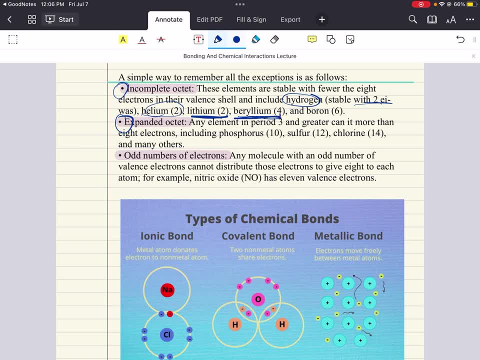 which is also very happy with just two valence electrons, Beryllium, which is happy with four valence electrons, And boron. Boron, which is happy with six valence electrons. These are, this is the first rule, all right. 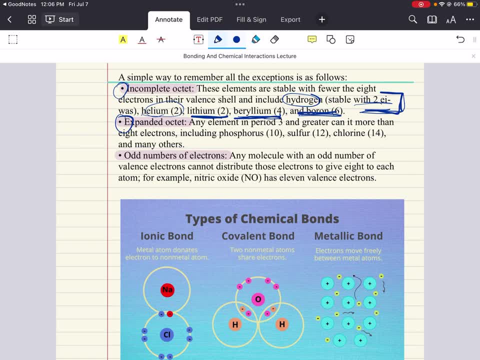 with examples of exceptions to the octet rule. all right, This is called the incomplete octet. We also have the expanded octet. Any element in period three and greater can hold more than eight electrons because of those d orbitals that are present. all right, 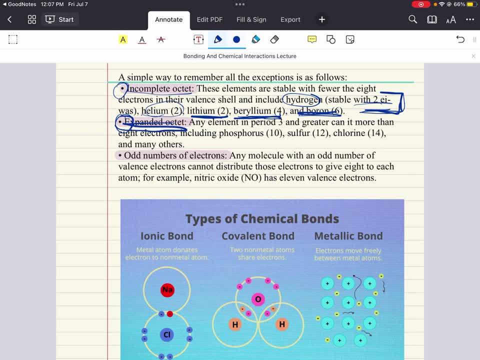 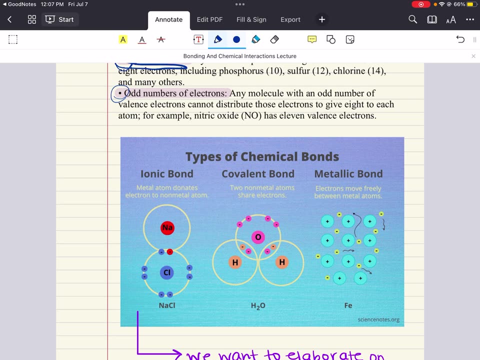 This is gonna include atoms like phosphorus, sulfur chlorine and many others that can have more than eight electrons to reach a stable configuration. And, last but not least, this third rule also helps us remember exceptions to this octet rule. It's called odd numbers of electrons. 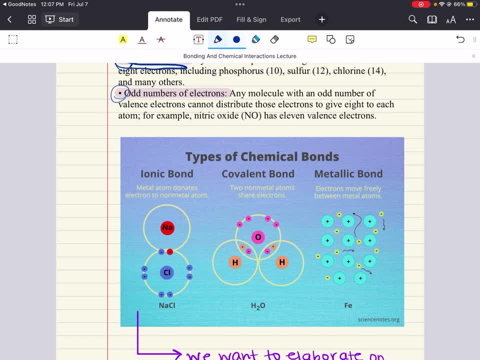 Any molecule with an odd number of valence electrons cannot distribute those electrons to give eight to each atom, All right. so, for example, nitric oxide has 11 valence electrons, all right. But it's happy with that configuration, all right. 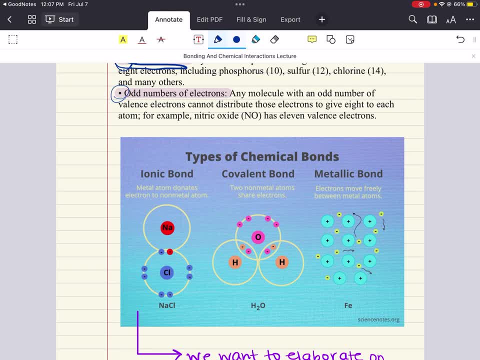 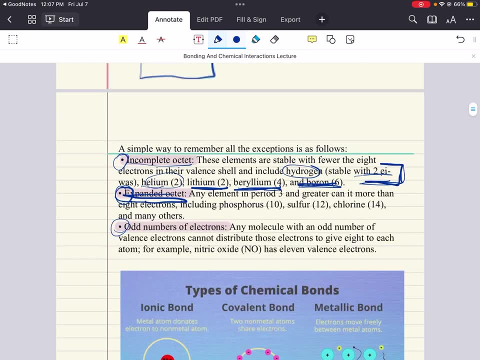 Now, another way to remember the exceptions is to remember the common elements that almost always abide the octet rule, all right. So what you can do is you can remember all the elements that follow the octet rule, all right, Or you can follow all the exceptions, all right. 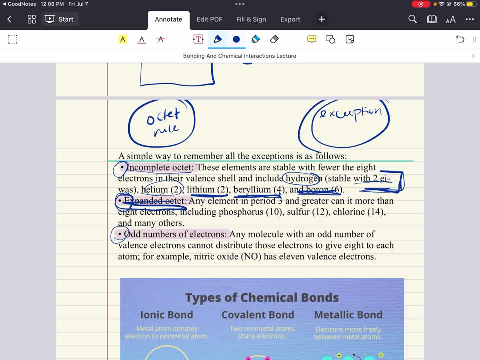 Either way, you'll know how to interact with different elements in regards to this. So what are the elements that follow the octet rule? That's gonna be carbon nitrogen, oxygen, fluorine, sodium and magnesium, all right. 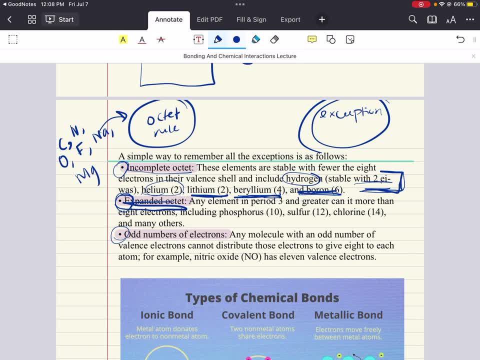 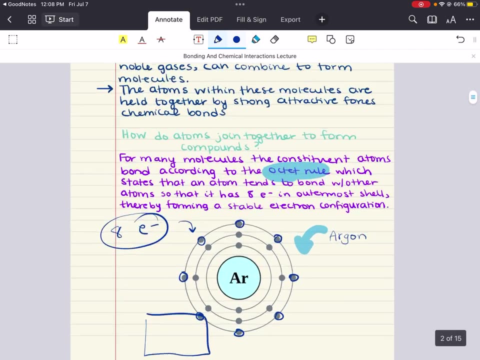 These are some of these elements that will follow the octet rule. Note that nonmetals gain electrons and metals lose electrons to achieve their respective complete octets. All right, so the octet rule is just a rule of thumb. that says for many molecules. 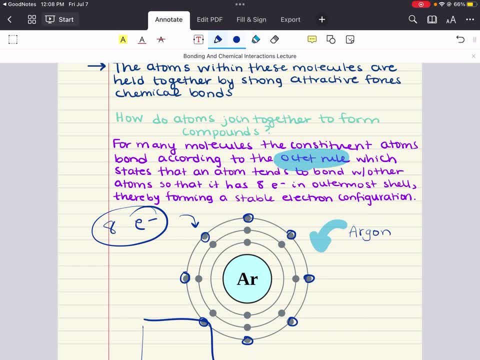 the constituent's atoms bond according to the octet rule, which states that an atom tends to bond with other atoms so that it has this eight electrons in its outermost shell, thereby forming a stable electron configuration that's comparable to noble gas configuration. The atoms that you should always remember. 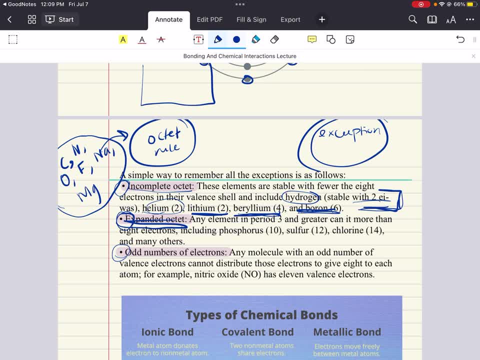 follow the octet rule. octet rule are carbon nitrogen, oxygen, fluorine sodium and magnesium. There are exceptions to this rule, of course, and the three rules that are gonna help you remember what atoms tend to expand beyond the octet rule. 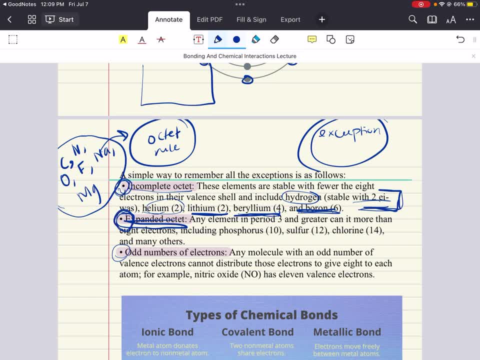 is the rule that's called incomplete octet, expanded octet and odd number of electrons. All right, fantastic. With that we can move into discussing the different types of bonds. All right, we have two distinct types that we're gonna focus on in this chapter. a great deal. 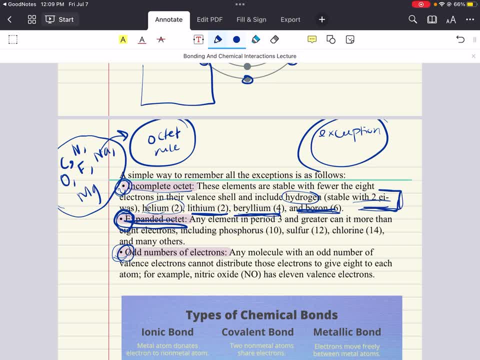 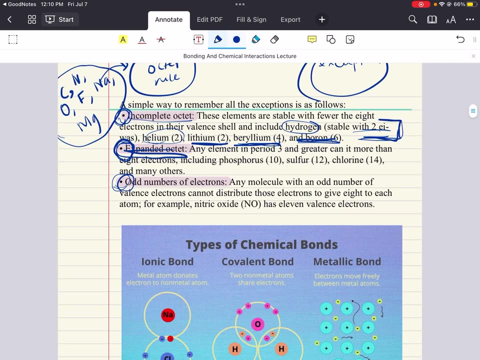 All right, that's gonna be ionic bonding and covalent bonding. In ionic bonding, one or more electrons from an atom with a low ionization energy, so typically a metal, are transferred to an atom with a high electron electron affinity, typically a non-metal. 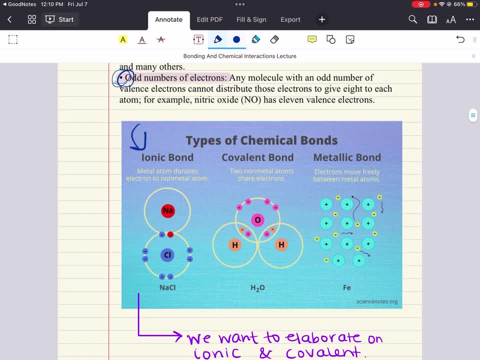 All right, so that's ionic bonding. Metal atom donates electrons to non-metal atom. What about covalent bonding? In covalent bonding, an electron pair is shared between two atoms, typically non-metals, that are gonna have relatively similar values. 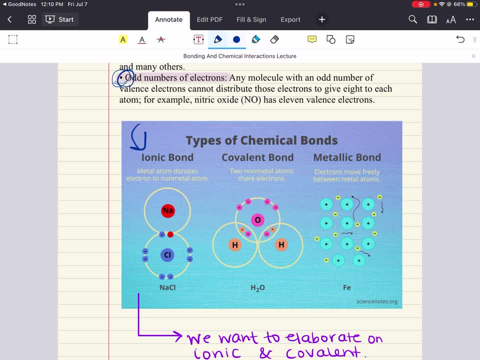 of electronegativity. The degree to which the pair of electrons is shared can be equally or unequally, and we're gonna elaborate on that shortly, all right. But in short, covalent bonding is two non-metal atoms that share electrons to some degree. all right. 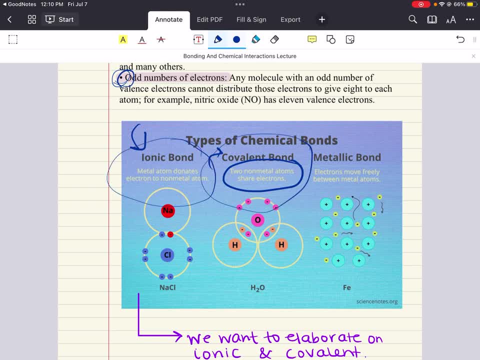 Now, these are the two main types of chemical bonds that we're gonna focus on tremendously in this chapter. I wanna take one second to make note of another type of bond called metallic bond. This is when we have electrons that are gonna move freely between metal atoms. 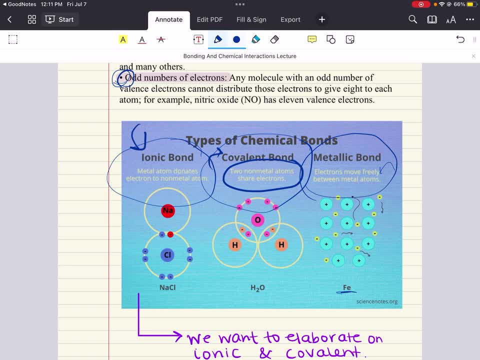 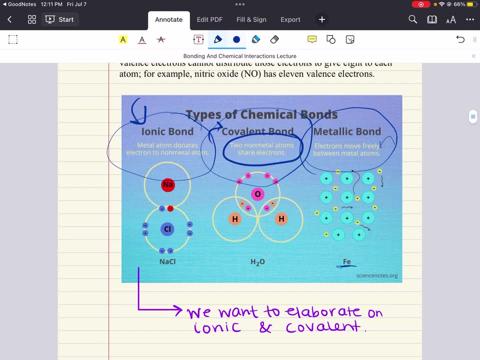 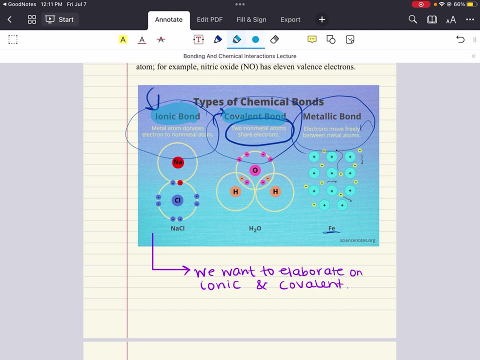 We're not gonna focus on this so much here in this chapter, all right, but it's important to know that there is this variety of chemical bonds. Now I want to take this information on ionic bonds and on covalent bonds and show you a flow chart. 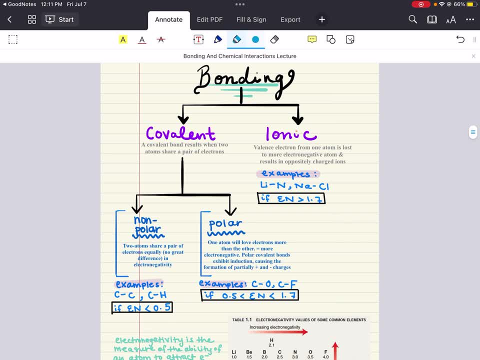 that can help us think about these different types of bonding. that's gonna allow us to ask a very important question. all right, We said there are two different kinds of bonding. Ionic bonding: this is when the valence electron from one atom is lost to a more electronegative atom. 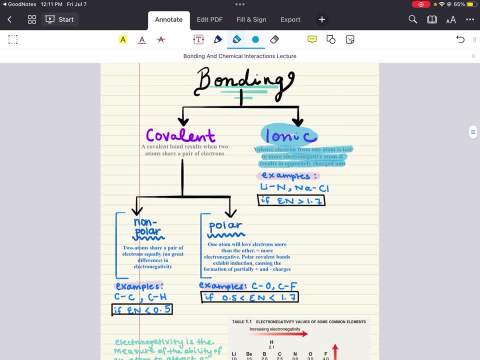 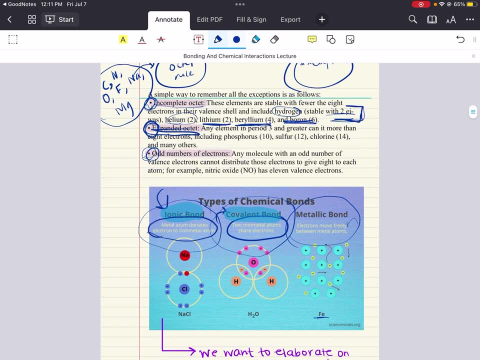 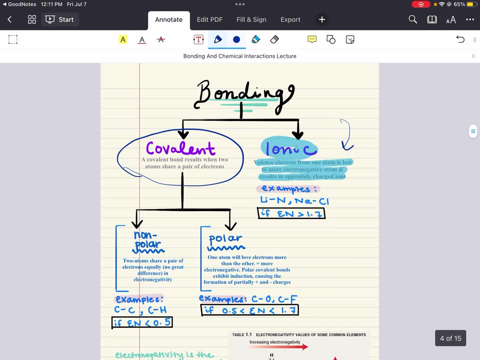 and it results in oppositely charged atoms. This is a more precise way of writing this definition. Metal atom donates electron to non-metal atom. all right, Then we have covalent bonding. This is the other variety of chemical bonding we're gonna talk about. 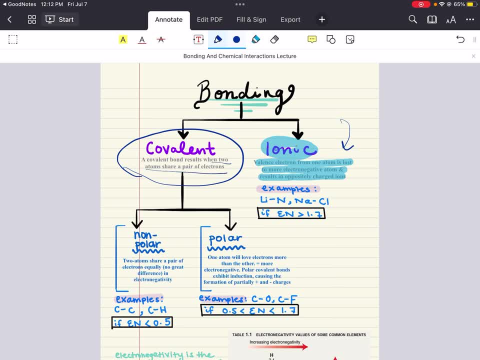 A covalent bond results when two atoms share a pair of electrons. Now, in covalent bonding, the degree to which the pair of electrons is shared can be of two varieties. The pair of electrons between two atoms that are forming a bond can be shared equally. 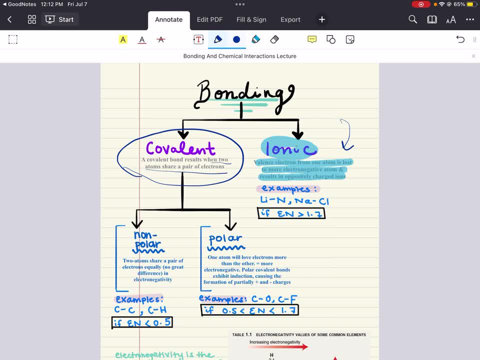 or unequally between the two atoms. Of course this determines the degree of polarity in the covalent bond. For example, if the electron pair is shared equally between the two atoms, then that covalent bond is non-polar. all right. 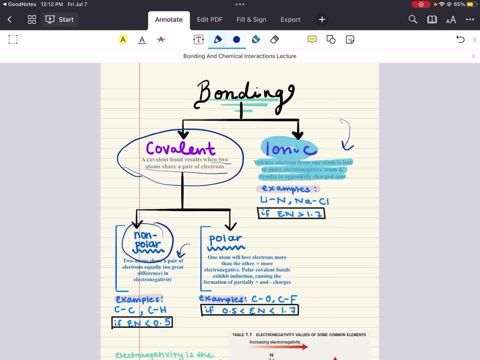 Non-polar is when two atoms share a pair of electrons equally. all right, What about if the pair is shared unequally? Then the bond is polar. Polar is when one atom will love electrons more than the other and thereby pull the electrons. 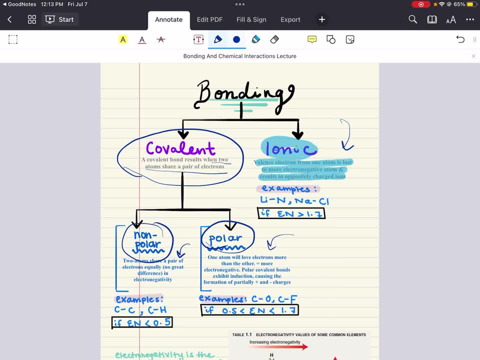 more towards one atom versus the other and the bond becomes polar. all right, Nonpolar, polar. two varieties of covalent bonding. Now this flow chart of different kinds of bonding: ionic and then covalent, and then the two varieties. 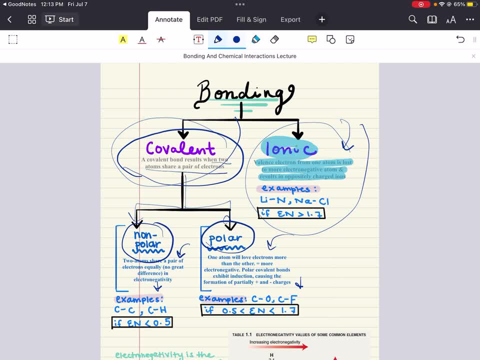 of covalent bonding: nonpolar covalent bonding. polar covalent bonding bonding. it allows us to ask a really important question, And that question is: well, what variable do we use to determine what kind of bonding is occurring? What's a precise way of? 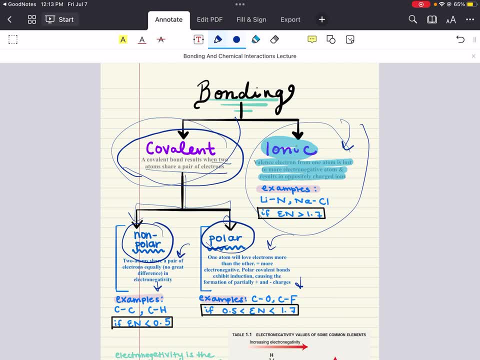 looking at two atoms that are forming a bond. What is a precise way of looking at two atoms that form a bond and being able to determine that that bonding is a ionic bonding, that that bonding is a covalent bonding, And then to probe even further and to say that that is a nonpolar? 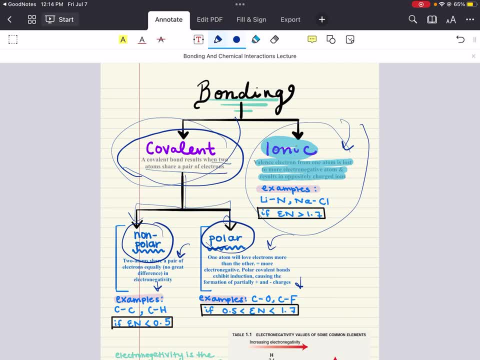 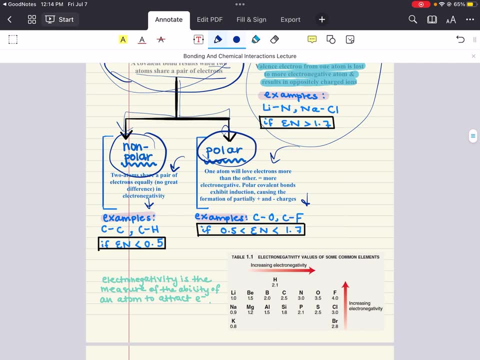 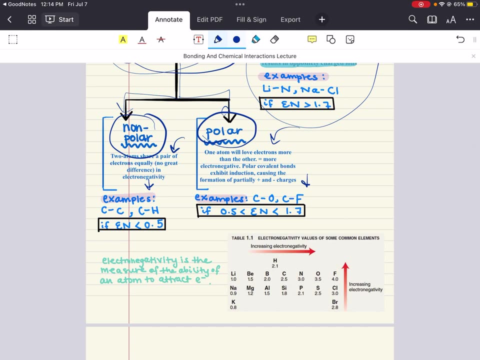 or polar covalent bond. What variable do we use to determine what kind of bonding is occurring? And the answer to that question is electronegativity. All right, electronegativity, This is the measure of the ability of an atom to attract electrons. Each atom has an. 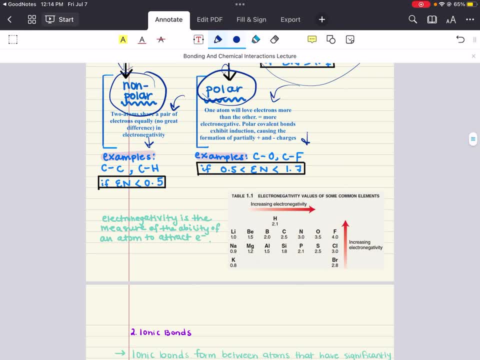 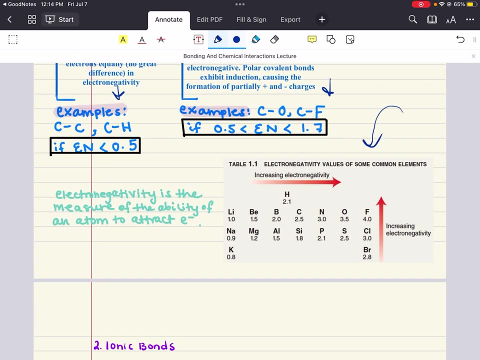 electronegativity, Electronegativity value, All right. And when two bonds are forming, when two atoms are forming a bond, the difference between their electronegativity values determines their bonding. Now, there are many different electronegativity scales. The Linus Pauling electronegativity scale is the one. 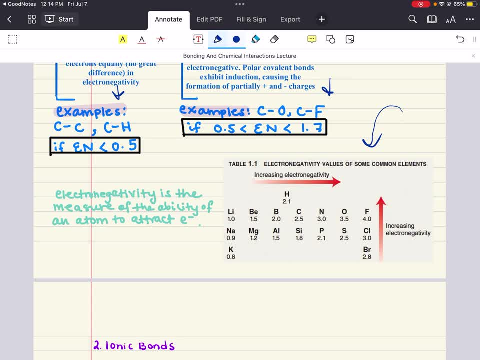 that you're going to commonly see used in MCAT books. It's what's shown here. All right, Here we see a table of electronegativity: Electronegativity values of some common elements. All right, You don't necessarily need to remember. 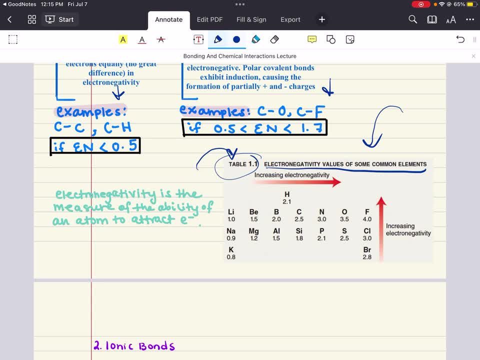 the values exactly. If you can remember the trends, you're going to be more than OK on the MCAT. Remember- we talked about this in the previous chapter- Going from left to right on a periodic table, the electronegativity values increase, And then going from bottom to top. 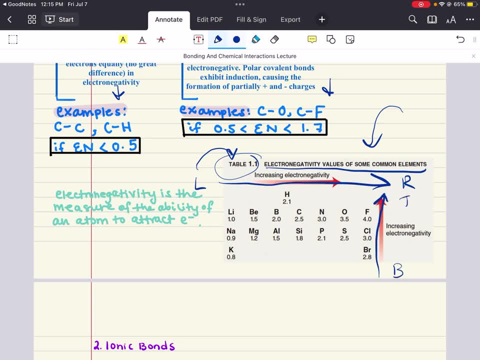 the electronegativity values also increase. All right, But let's use this table to look at a couple of examples. All right To then discuss ranges that allow us to determine if a bond is nonpolar, covalent, polar covalent or ionic. All right. 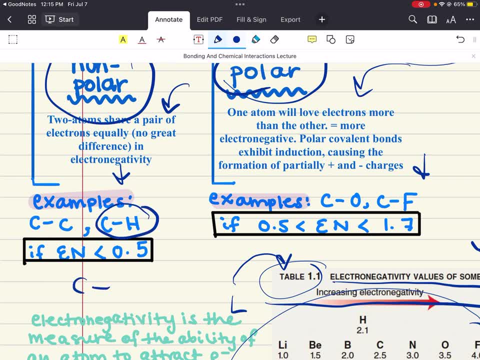 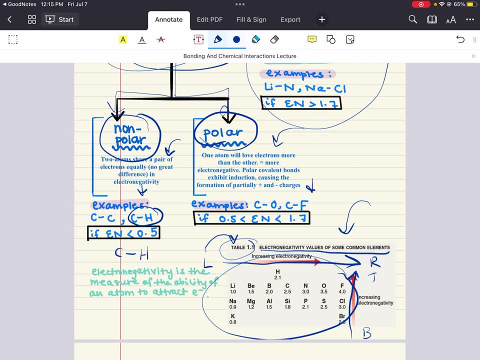 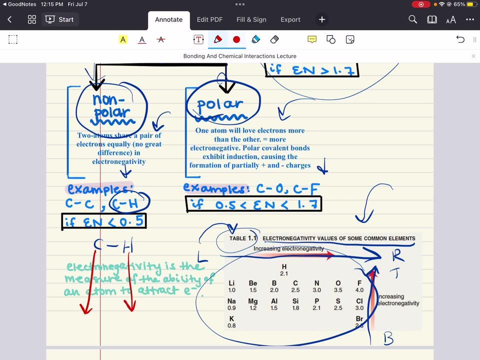 So, for example, let's say we're looking at a carbon-hydrogen bond. We want to determine what kind of bonding is occurring between this carbon and this hydrogen. How do we accurately determine what kind of bonding is happening between this carbon? We're going to get those electronegativity values of carbon and hydrogen. Carbon has an 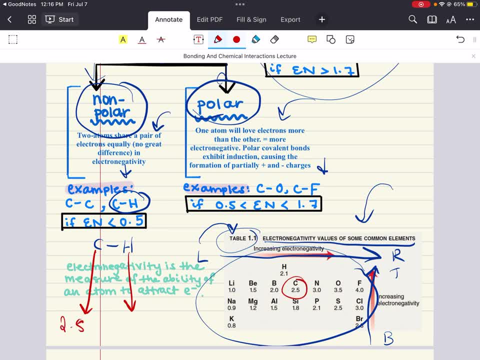 electronegativity value of 2.5.. Hydrogen has an electronegativity value of 2.1.. We're going to take the difference between these two atoms. All right, We get 0.4.. If the difference between 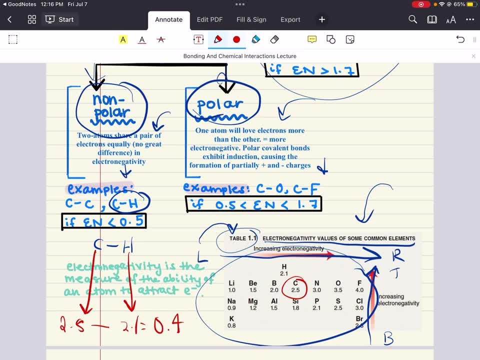 electronegativity values of the two atoms forming a bond is less than 0.5, then what we have here is a nonpolar covalent bond. This is a nonpolar covalent bond because the difference in electronegativities is 0.4,, which is less than 0.5.. All right, Cool, So that is how we can determine. 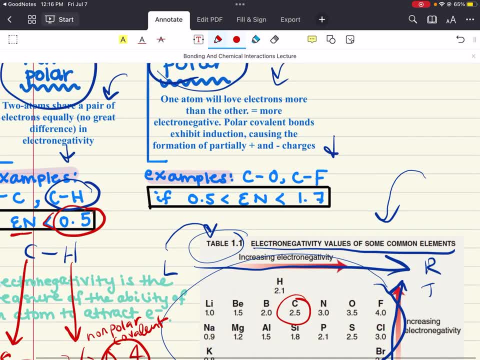 nonpolar covalent bonding. What about polar covalent bonding? Let's look at carbon-oxygen as an example. Carbon has an electronegativity value of 2.5.. Hydrogen has an electronegativity value of 3.5.. The difference between these two. 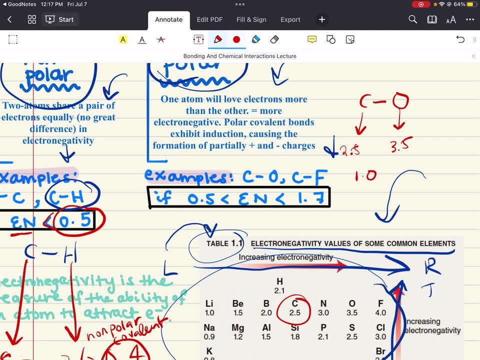 all right. the absolute difference, if you will all right, is 1.. 3.5 minus 2.5 is 1.. All right, This falls in the range of 0.5 and 1.7, which is the definition of a polar covalent bond. 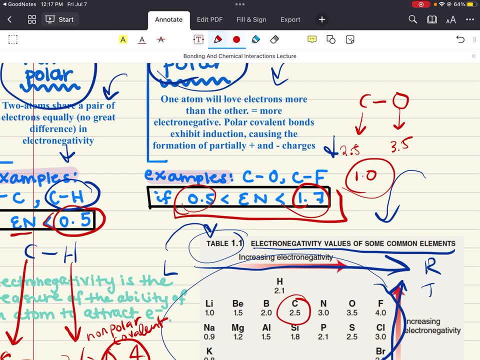 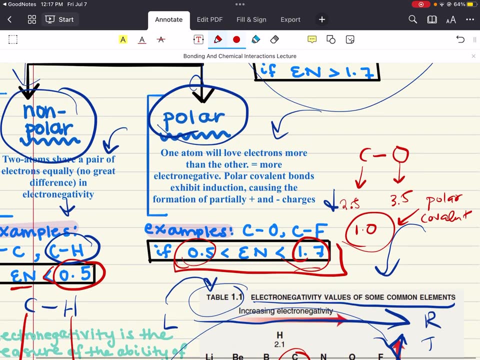 If the difference in your electronegativity, all right, falls anywhere between 0.5 and 1.5,, this is a polar covalent bond, Fantastic. Now what if the electronegativity difference is greater than 1.7? All right. For example, let's look at sodium chloride. Sodium has an 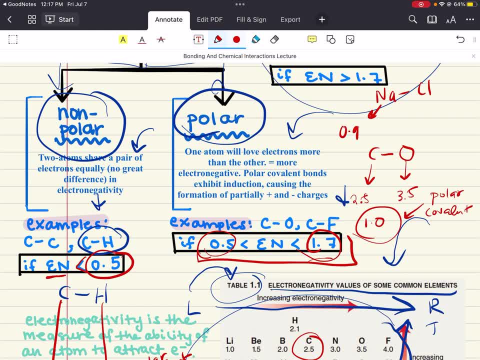 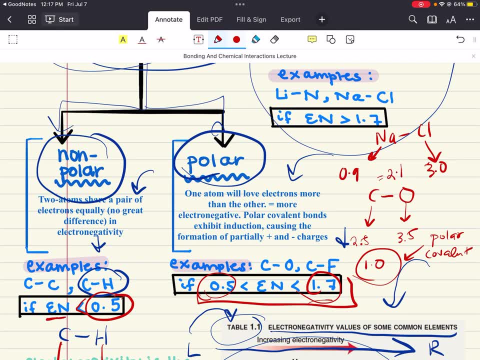 electronegativity value of 0.9.. Chloride has an electronegativity value of 3.. The difference here is going to be 2.1, which is much greater than 1.7.. Greater than 1.7 electronegativity. this is an ionic bond. All right. What that means is: 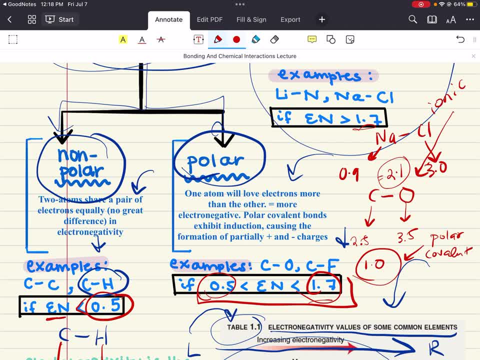 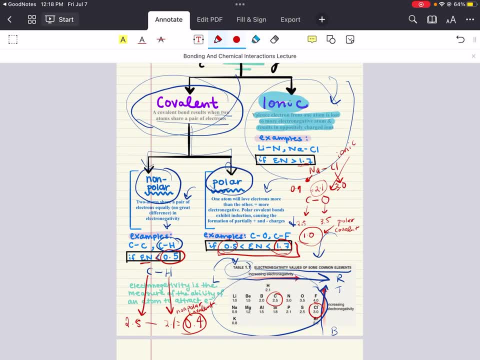 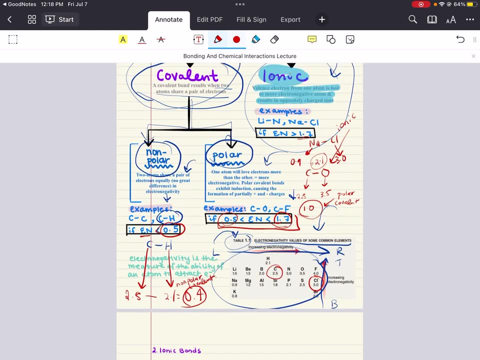 one of these atoms is going to donate an electron to the other atom, that is going to form an ionic bond. So this is how we can use electronegativity difference to determine whether a bond between two atoms is ionic, nonpolar or polar. All right, 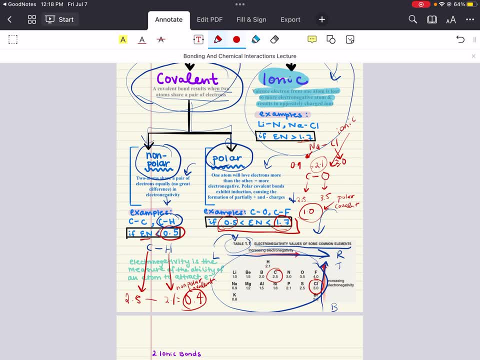 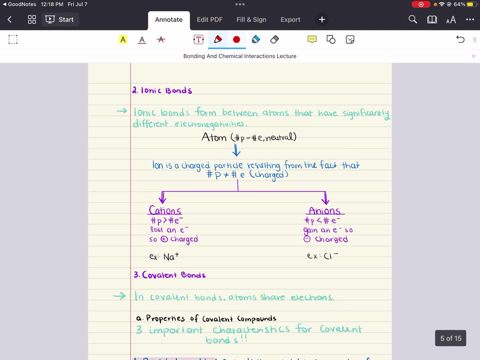 Now that we cover our first objective, we've broadly discussed different types of bonding- ionic and covalent, particularly All right- And we've also discussed the octet rule and the exceptions to the octet rule. We are now able to move into our second objective, which is a focus. 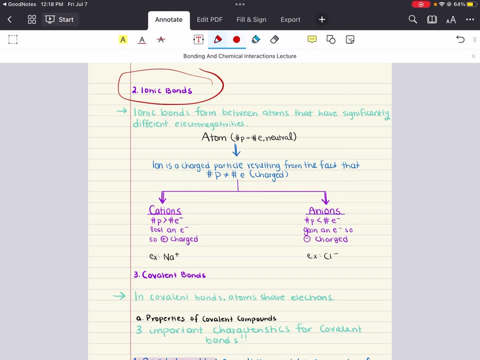 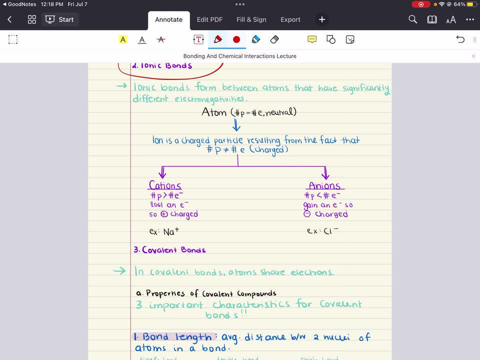 on ionic bonding: All right, Ionic bonds. these form between atoms that have significantly different electronegativity. All right. And we've also discussed the octet rule and the exceptions to the octet rule. We are now able to move into our second objective, which is a focus on 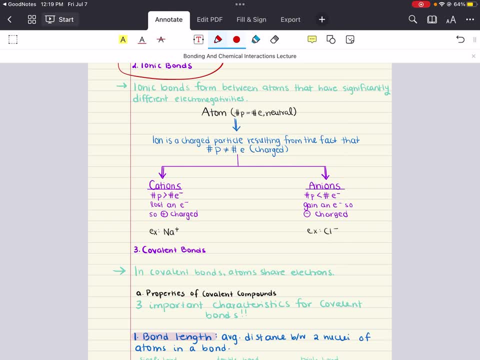 ionic bonding All right, And we've also discussed the octet rule and the exceptions to the octet rule. We are now able to move into our second objective, which is a focus on ionic bonding. All right. We have significantly different electronegativities and that is how you determine if a bond between 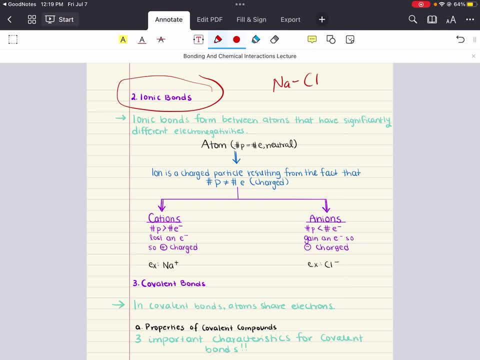 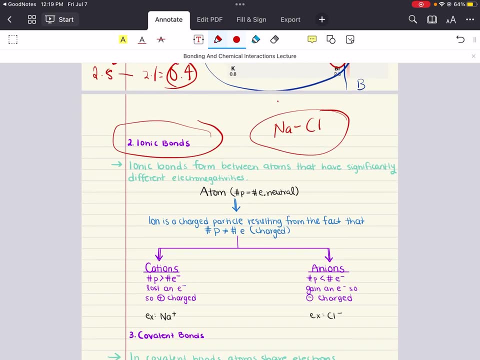 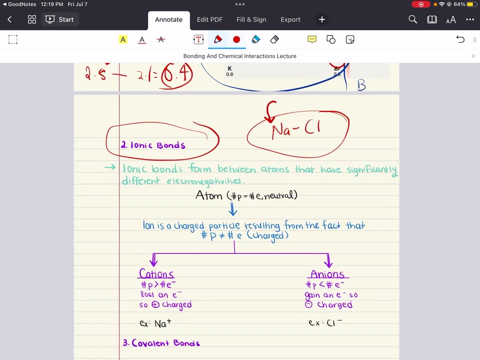 two atoms is ionic or not. Now, when you've determined that this is an ionic bond, what does this mean for us? This means that the atom with the lesser value of electronegativity, which will be our sodium, is going to donate. 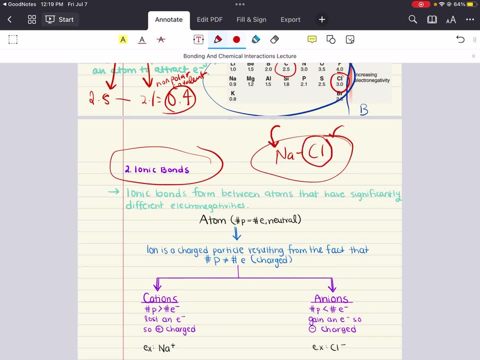 an electron to our atom with greater electronegativity. So our sodium, which has, by the way, only one electron in its outermost shell, it's going to donate that electron to chlorine, which has seven electrons in its outermost shell. So sodium donates that electron. 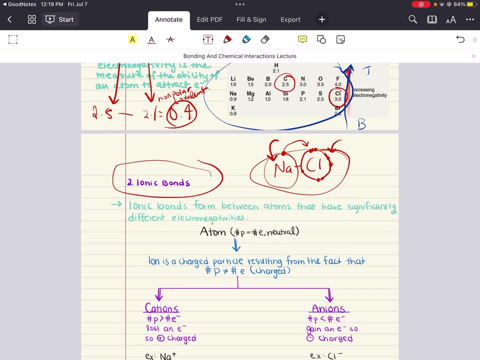 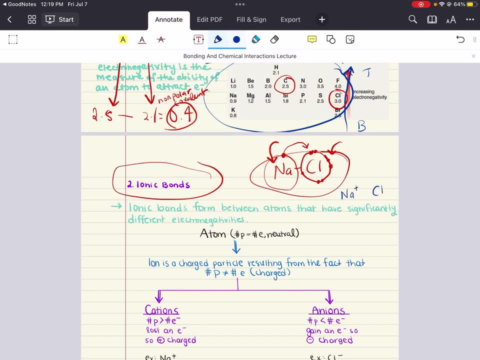 to chlorine. Now, sodium has lost an electron, so it's going to have a positive value associated with it, And chlorine has just gained an electron, so it's going to have a negative value associated with it, because now it has one more extra electron- The atom that loses the electron. 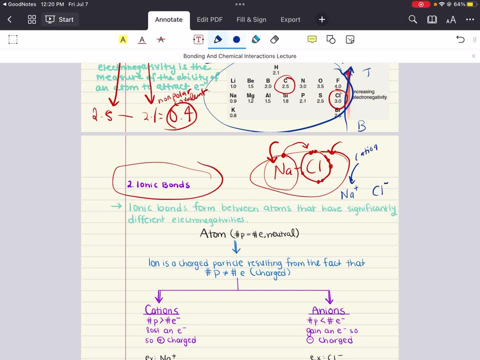 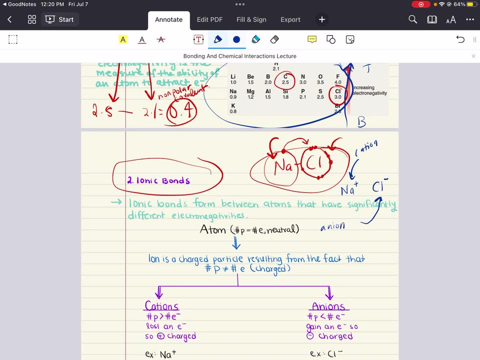 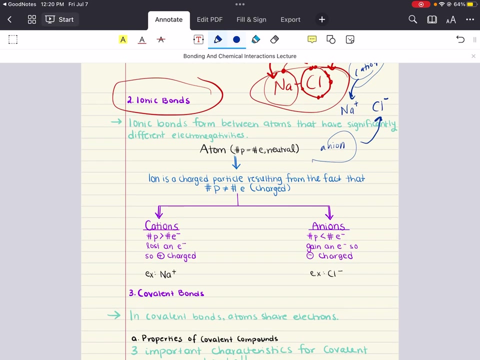 becomes the cation and the atom that gains an electron is known as an anion. The ionic bond, essentially, is just the result of an electrostatic force of attraction between these oppositely charged ions, Between the cation and the anion. So the ionic bond is just the result of an electrostatic force. 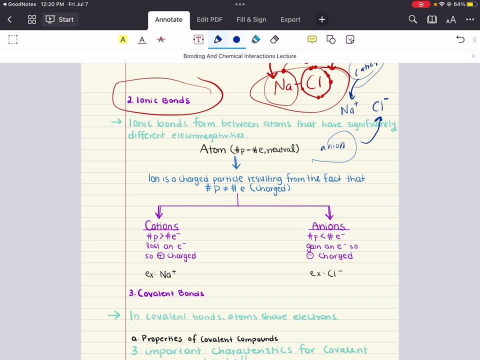 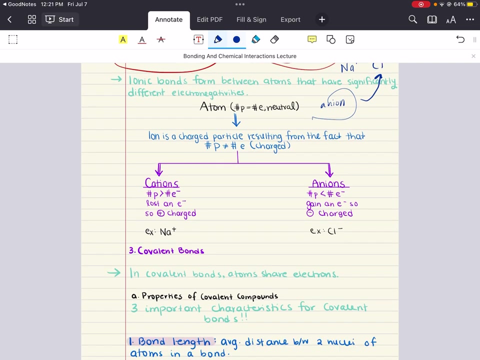 of attraction between the opposite charges of these ions. Electrons are not shared in an ionic bond. They're donated from one atom to another. For this electron transfer to occur, the difference in electronegativity must be greater than 1.7 on the Pauling scale, like we discussed. Now to remember, all right, 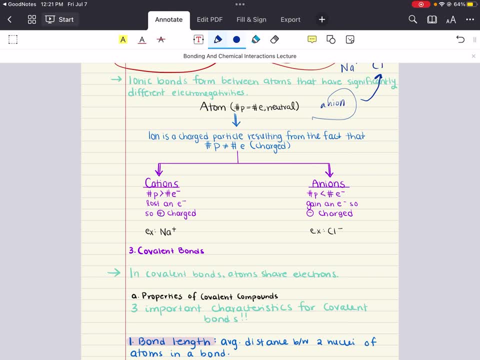 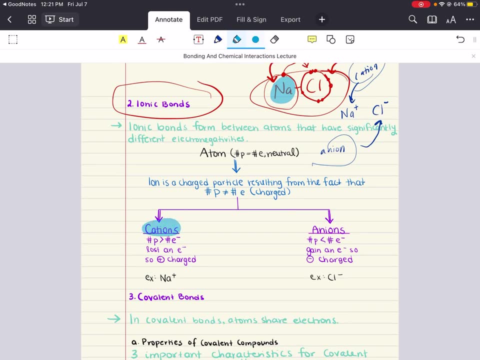 remember that metals lose electrons to become cations. Sodium is a metal. It loses electrons to become a cation. All right, cation now has a greater number of protons than it has number of electrons, which is why it has a positive charge associated with it, which is why we gave sodium. 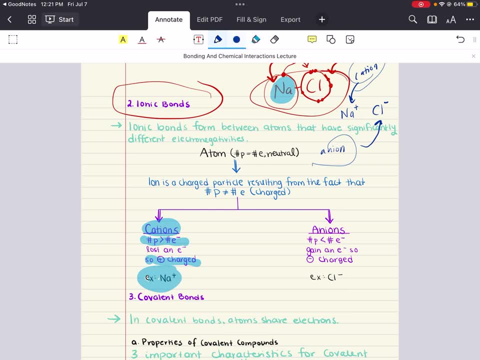 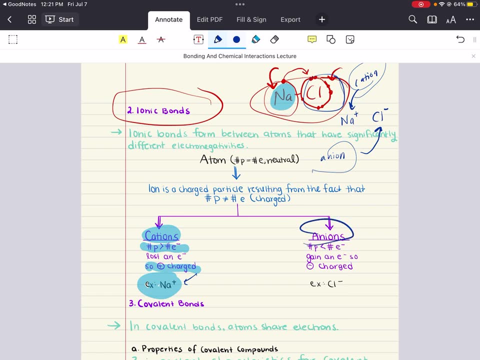 that positive Symbol here. All right, Nonmetals like chlorine. Chlorine's a nonmetal. It gains electrons to become anions. Now it has greater number of electrons than it does protons, which is why it has a negative charge associated with it. All right, And so now you have sodium. that's your cation. 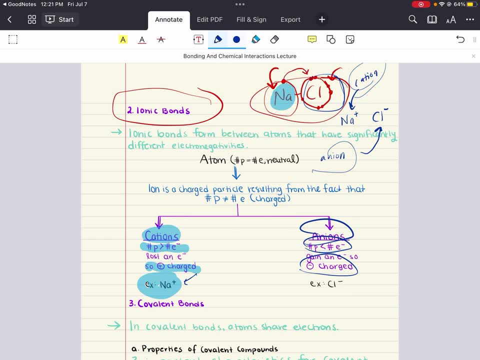 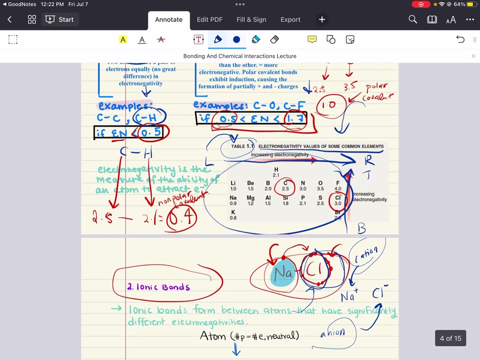 Chlorine, that's your anion. All right, They have an ionic bond. Notice how chlorine gained that last electron. So now it has noble gas configuration, right, Stable noble gas configuration or noble gas-like configuration? Now again, the MCAT won't expect you to memorize this Pauling scale, for 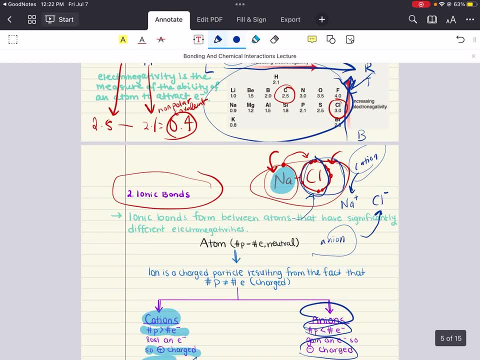 electronegativity, but recognize that ionic bonds are generally formed between a metal and a nonmetal, For example alkyl and alkaline earth metals. that's where the ionic bonds are. So, for example, the ionic bonds are generally formed between a metal and a nonmetal. So 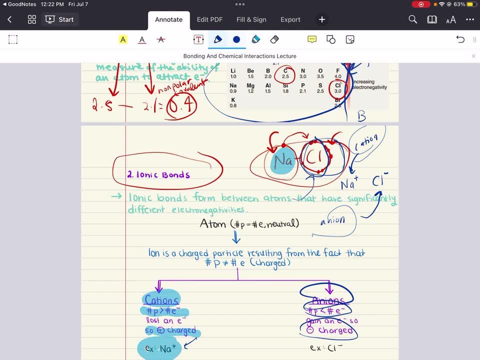 for example, alkyl and alkaline earth metals. that's where the ionic bonds are. So, for example, group 1A and group 2A: all right, they readily form ionic bonds with halogens. group 7A, The 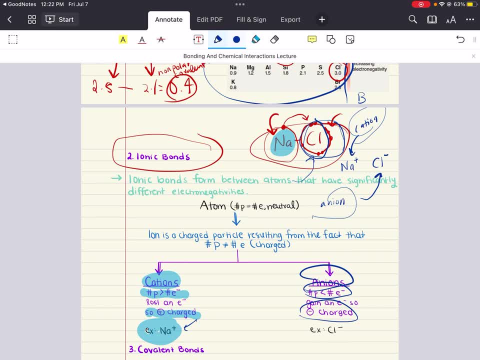 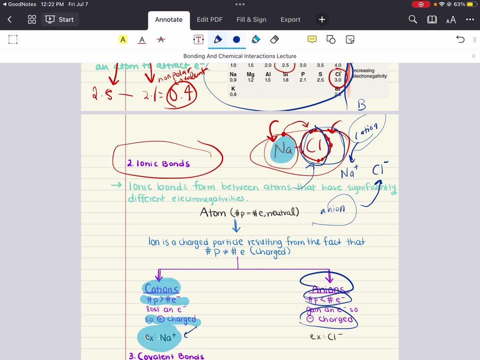 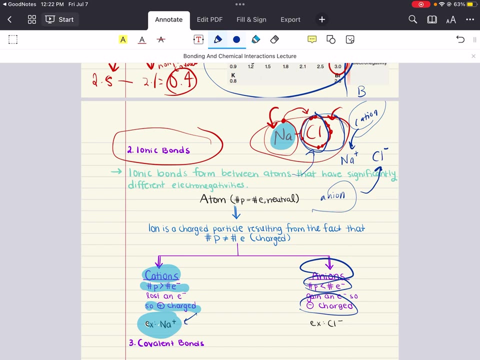 atoms of the active metals loosely hold onto their electrons, whereas the halogens are more likely to gain an electron from those alkali and alkaline earth metals to try and complete their valence shell. The difference in bonding behavior for these classes of elements. 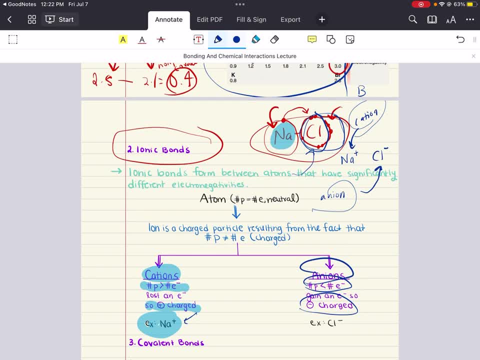 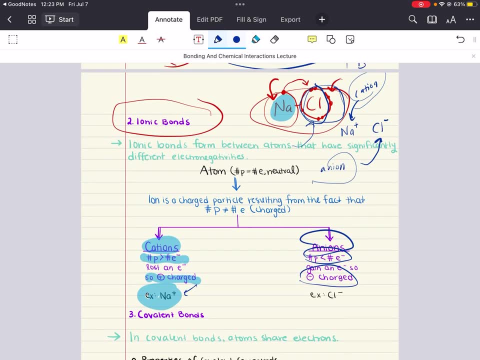 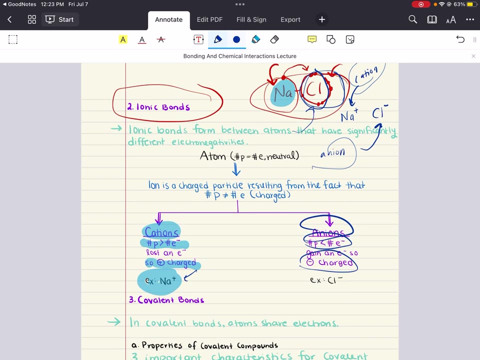 and of course, the difference in electronegativity values explain the formation of ionic compounds, like we've done here with sodium chloride as an example. Now one note I want to make, because of the strength of the electrostatic force between 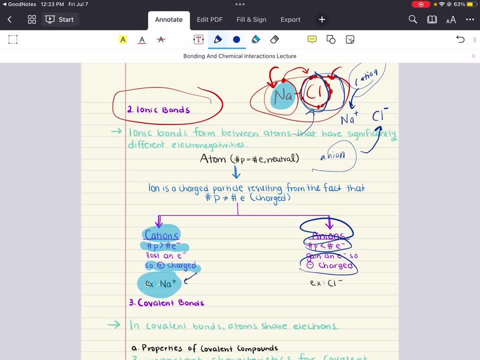 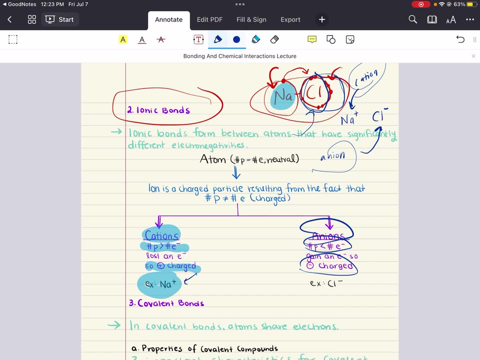 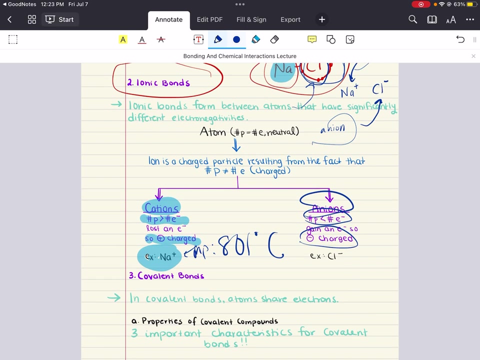 the ionic constituents of a compound like sodium chloride ionic compounds. they tend to have a very high melting and a very high boiling point. For example, the melting point of sodium chloride is 801 degrees Celsius. Also, many ionic compounds dissolve readily in aqueous and other polar solvents solutions. 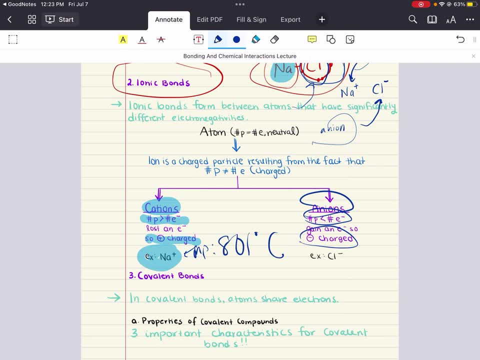 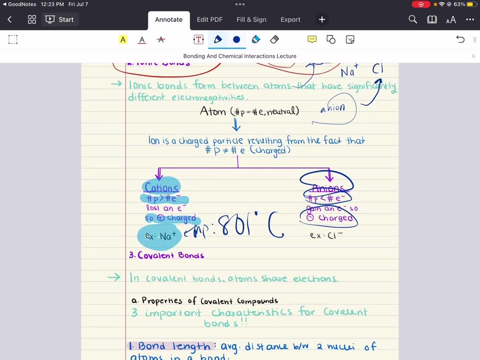 and in the molten or aqueous state they tend to be very good conductors of electricity. In the solid state the ionic constituents are varied and other waiting states like topography of the compound. they form a crystalline lattice that consists of repeating positive and negative. 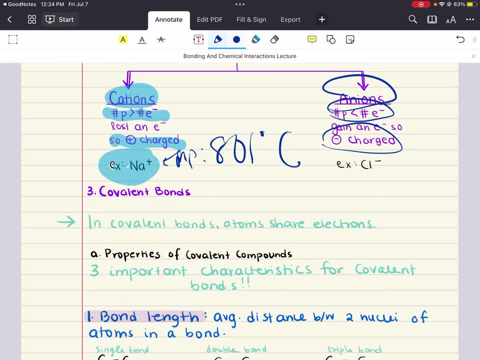 ions. So what does an ionic sodium chloride structure look like? Well, the crystal lattice structure of sodium chloride looks like repeating units of sodium and chloride. sodium and chloride all right formed in this crystal lattice structure, repeating all right, And it kind of forms like: 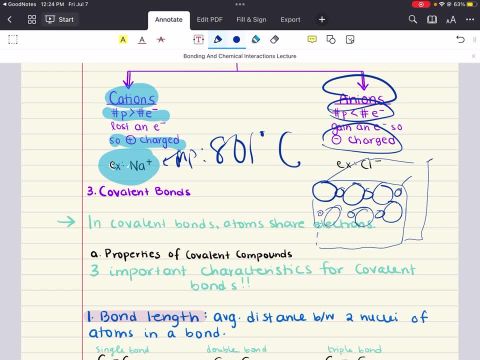 some sort of crystal lattice structure that's associated with the compound. all right, With this arrangement, essentially the attractive forces between the oppositely charged ions are going to be maximized and the repulsive forces between ions of like charges are going to be. 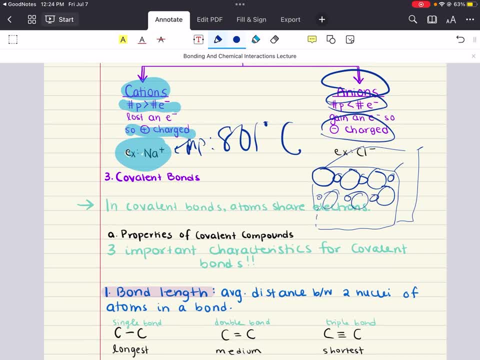 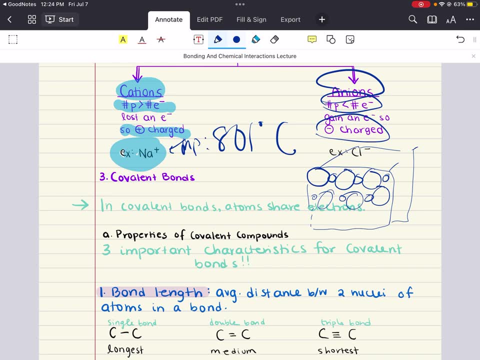 minimized- Fantastic. So with that we have covered ionic bonds. Remember: metals lose electrons to become cations, Ions- positive ions- And nonmetals gain electrons to become anions- negative ions. All right, fantastic. We're going to end this video here. Next time we're going to move into our third. 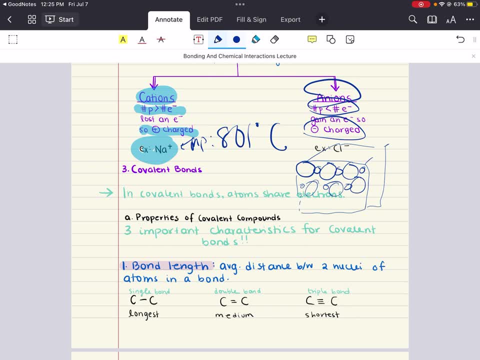 objective, which is about covalent bonds. All right, here we're going to talk about how do we define covalent bonds. We're going to discuss properties of covalent bonds. We're going to discuss how we can draw Lewis structures. We're going to discuss VSEPR theory.